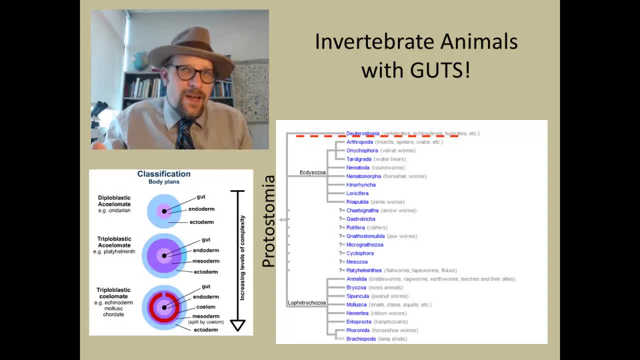 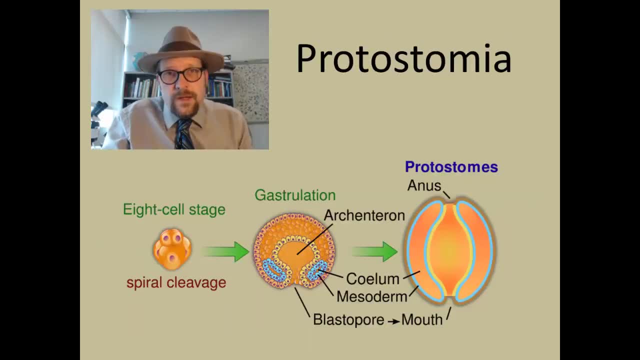 lack a coelom, but they also lack much of a fossil record, so we are not going to talk much about them in this class. The origin of a gut was likely developed twice in the early evolutionary age In protostomes, which include many invertebrate groups, including insects and the group 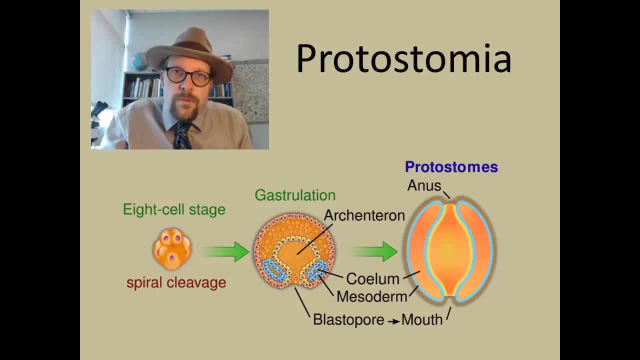 that we are going to talk about today, the bryozoans. the mouth is formed from the blastopore. This is the original opening during the gastrulation stage of the early embryo, while the anus becomes a separate later opening. This is in contrast to deuterostomes, which include: 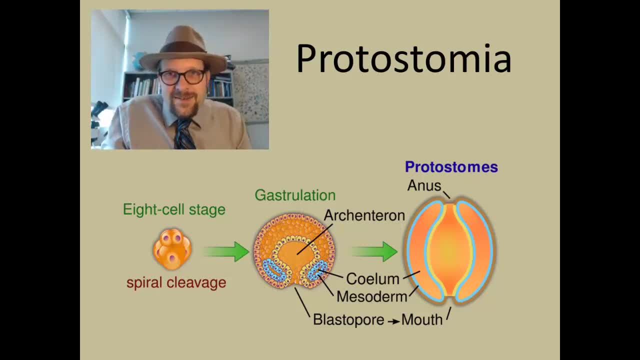 us humans, And it also includes the anus. It also includes echinoderms, the starfish, and in us starfish the initial opening develops into the anus, and our mouths are a secondary development in the early embryo, often surrounded by mesoderm cells which later go on to form our brains and other things. 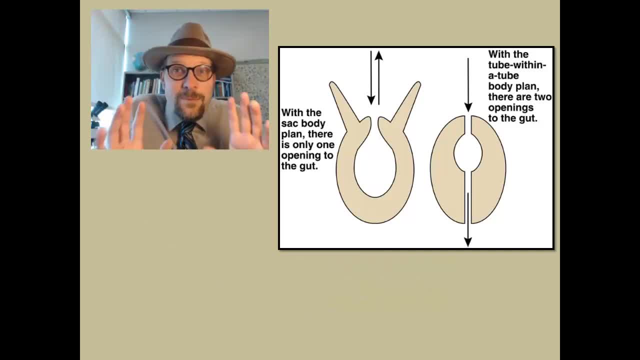 The gut tube is a pretty important innovation and it is not surprising that it originated twice. Let's face it. Having an orifice that food goes in And then is digested And then passed out into a separate opening is a really nifty idea. 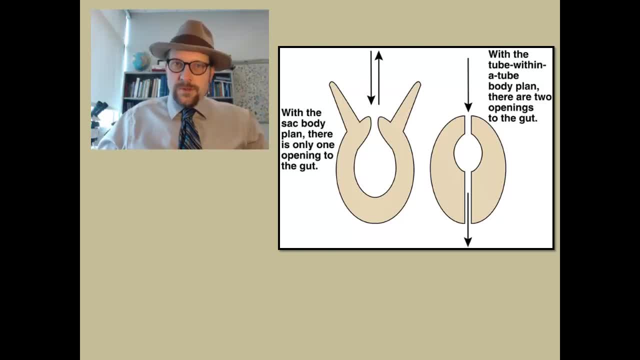 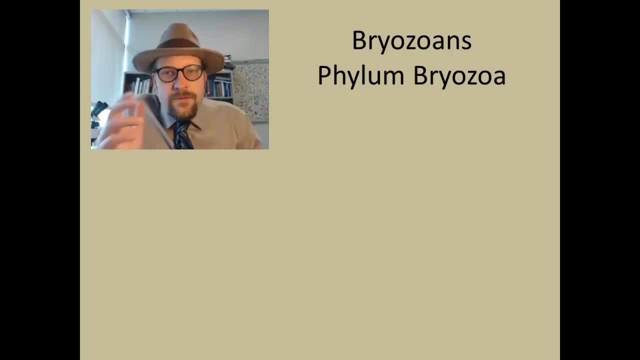 Digesting can be slow. You can keep the food coming down the tube, Which means you can grow faster. Alright, so let's talk about the first group of gut invertebrates, the bryozoans, the phylum bryozoa. 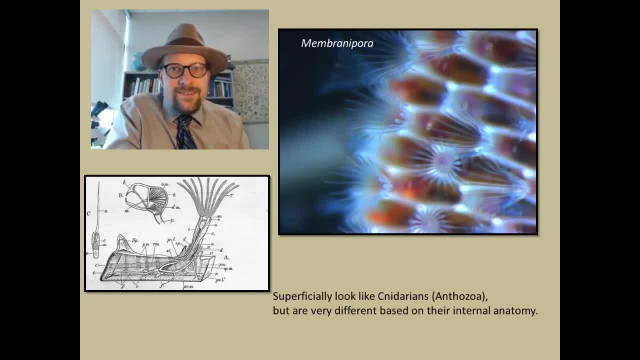 Now, the first thing you will notice about the bryozoa is that they superficially look like the cnidarians, like the anthrozoa, the sessile corals that we previously talked about, And they are not the same as the bryozoans. 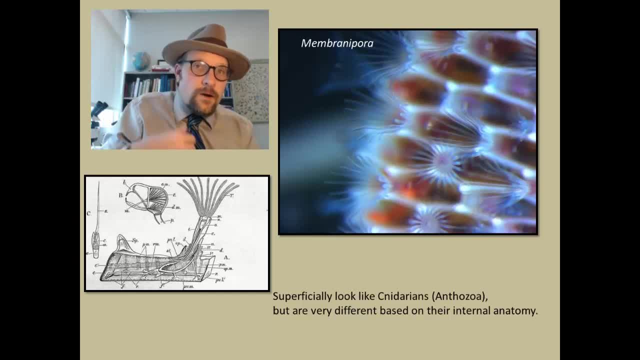 The bryozoans are the same as the cnidarians. They are not the same as the bryozoans. They are sessile colonial organisms and they live in the water. However, if you look closely, they are also unlike cnidarian corals, because these bryozoans 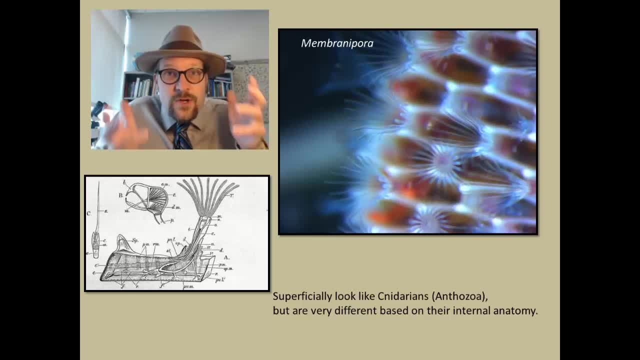 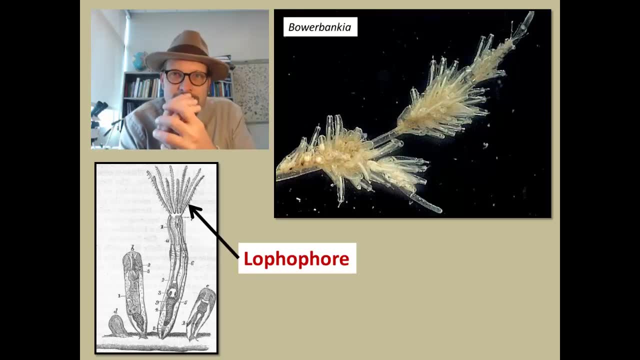 have digestive guts. they are digestive gurus. One of the important other features of bryozoans is a lofophore. This is a specialized food gathering organ that extends out of a tube or chamber and it can actively grab particles of food floating in the water and it brings it down to the 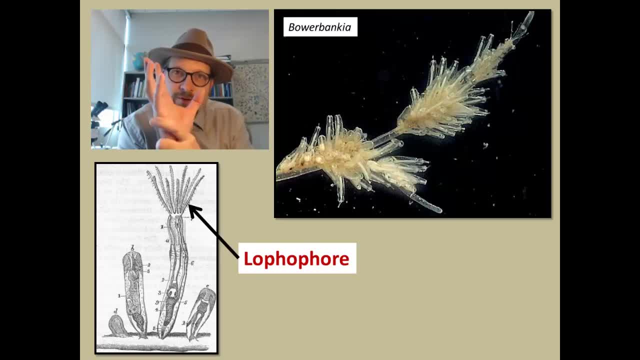 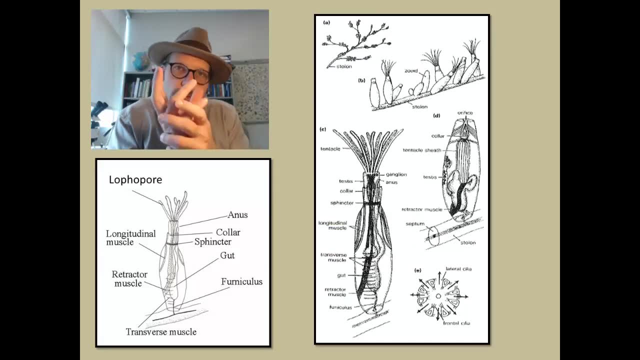 mouth. This lofophore is a shared trait that is also found in brachiopods, and we will discuss those in lecture 18.. Now, the lofophore pulls food into the mouth, which then passes through a narrow gut tube. 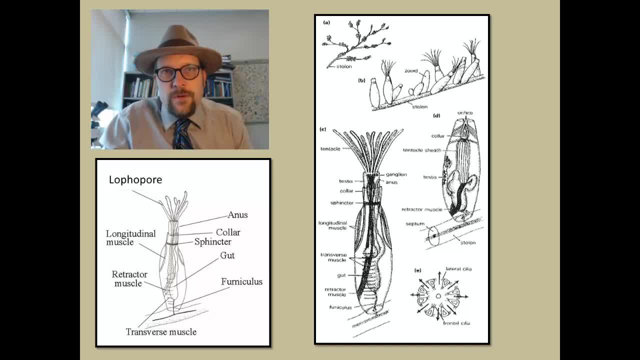 which then opens up to expel the undigested food and waste, which is actually just peripheral to the lofophore, To the mouth Right there. So the gut tube is actually u-shaped like that u-shaped loop. So the anus head and the mouth are pretty close together but they have separate openings. 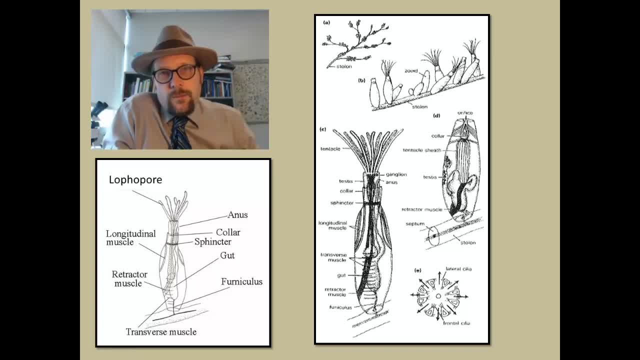 The lofophore also has one big difference when we compare it to the cnidarians, the true corals. It has a muscle that allows the lofophore to be retracted into the chamber. This is a pretty amazing specialization because this muscle tissue that retracts the 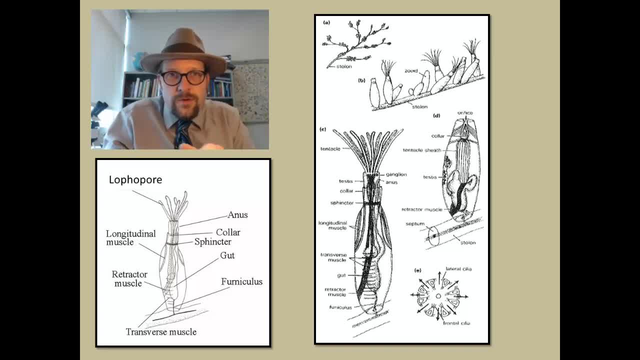 lofophore prevents it from being eaten or damaged when a predator comes swimming nearby. There is a sphincter muscle that closes the opening in some of these guys. that makes it very difficult for predators to eat these colonial creatures. Other types of bryozoans can close up these chambers with lids. 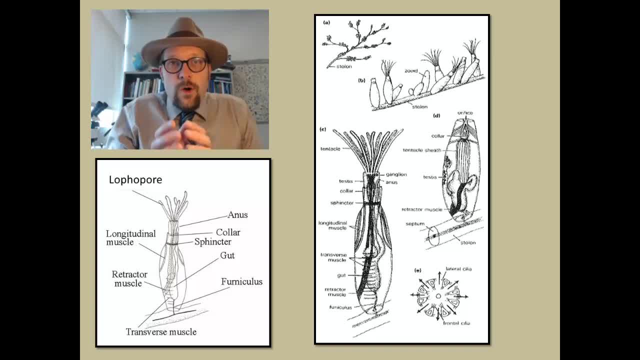 So what are the different types of bryozoans? Well, the first one is the bryozoan. The bryozoan is a very common species. It can open, back up and release the lofophore by inflating the ceclum which, through hydrostatic 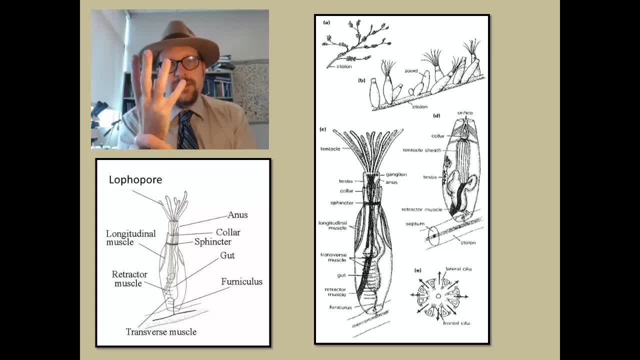 pressure extends the lofophore again. This arrangement of hiding away and coming out means that bryozoans can have sensory cells that trigger the reaction, to pull in Light sensing organs Or even sensing movement in the water that might indicate a predator nearby. so they 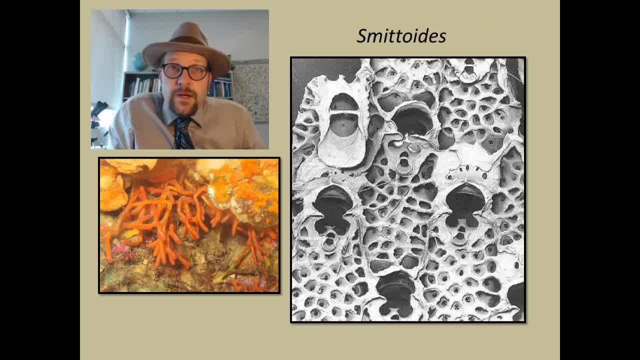 have that action to help them survive. Each pod is called a zooid and they are attached to each other in close association. Some bryozoans, like the living smetodes, have specialized zooids which change with ontogeny. 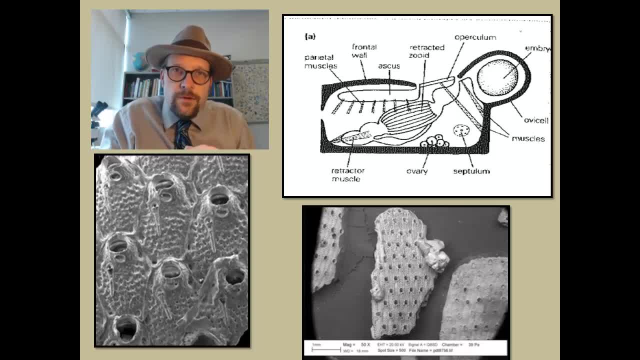 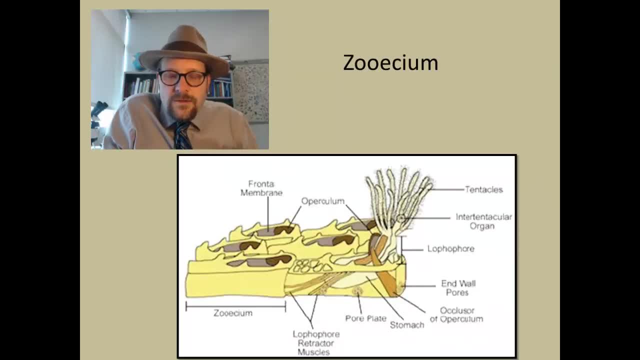 They can also have specialized chambers called ovocells, used for developing fertilized eggs into larvae. The calcified zooid skeleton is called a zoacum, and these zoacum are what are preserved in the fossil record. Some bryozoans have a hinged door for the opening called a reperculum, which, as we will, 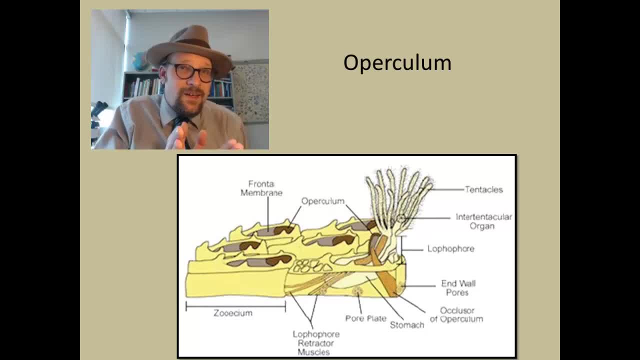 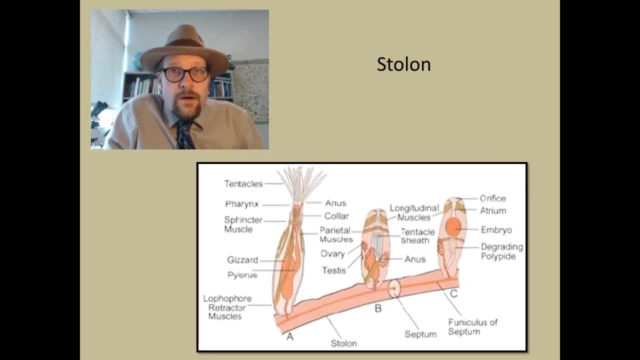 see with brachiopods could be related to the two sides of the shelled invertebrates. Bryozoans grow in close association with each other, often connected by structural walls of the zoacum Or, like in the case of brown banyans. 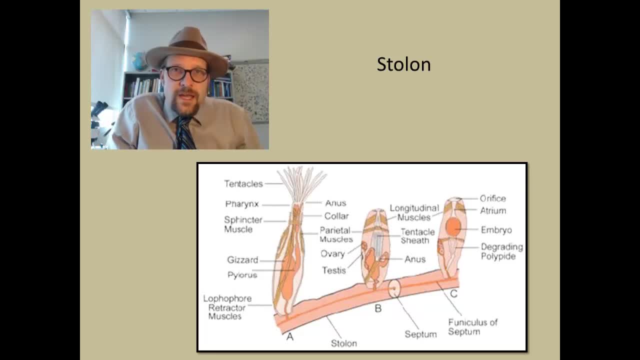 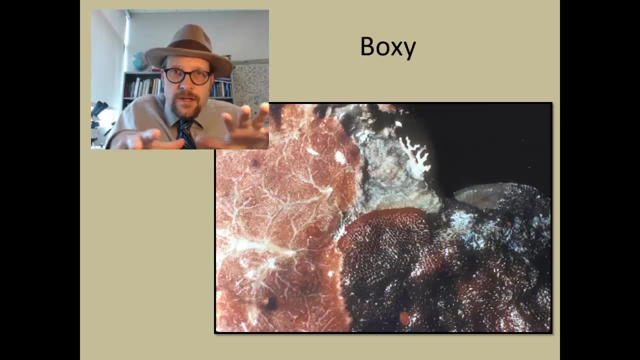 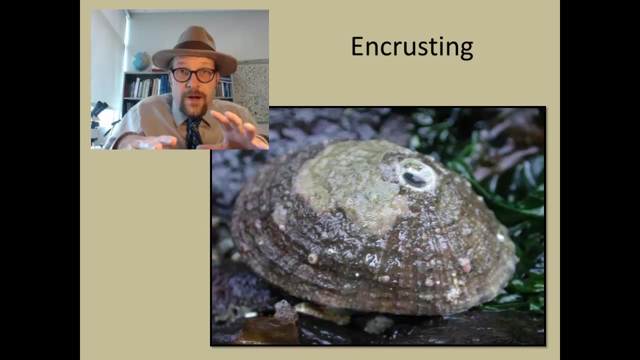 In the case of a brown bancheri, a stolum, which is a branching structure somewhat resembling branches on a plant Growth in bryozoans can be boxy in shape, they can form fan or feather shapes. they can be encrusting. they can grow on other animals, plants or even hard rocks. 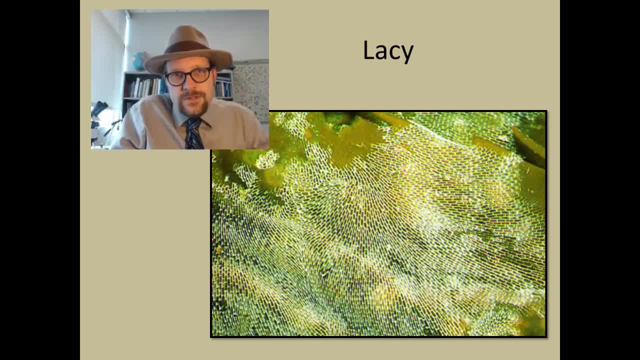 They can form pretty lacy textures as they grow out, secreting a calcium carbonate skeleton- In the case of brown bancheri, a stolum, which is a branching structure somewhat resembling branches on a plant. Or, like in the case of brown bancheri, a stolum, which is a branching structure somewhat. 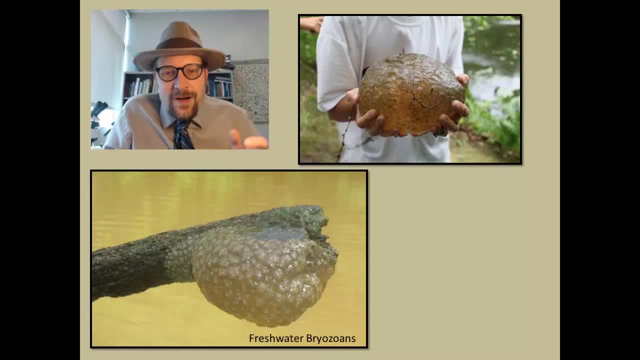 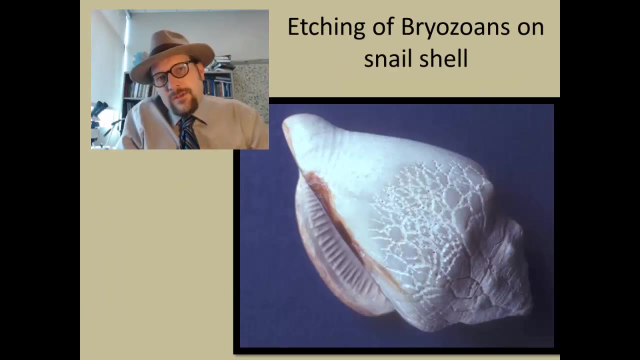 secreting a calcium carbonate skeleton, Sometimes in freshwater bryozoans. they form these big gelatinous balls that are found in freshwater rivers and ponds of colonies of bryozoans. Evidence of bryozoans are common in the fossil record because they can also etch into other. 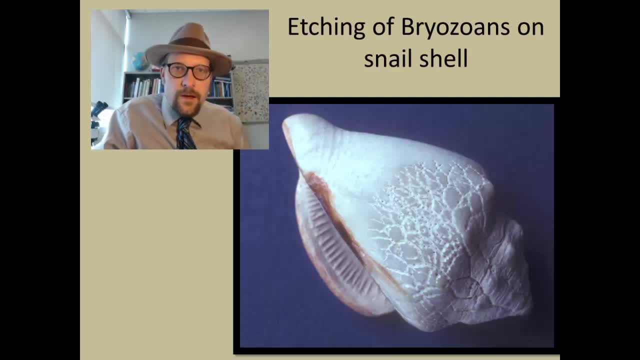 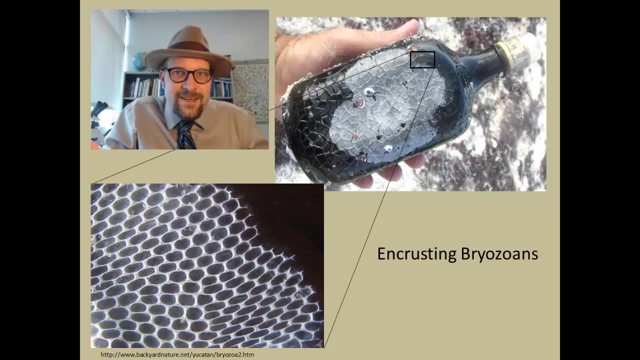 shelled organisms, such as this example of a snail shell, where you see little pits formed by encrusting bryozoans. Bryozoans can even encrust on trash that is left in the ocean. This encrusting nature of bryozoans means that we have an excellent fossil record, since 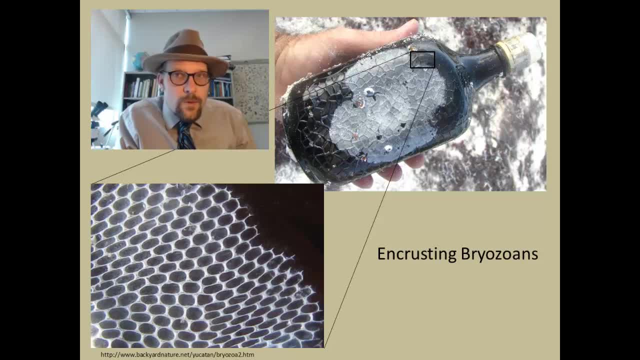 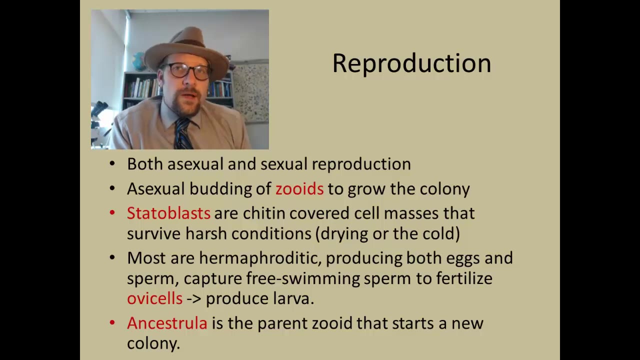 they rarely grow on hard substrates and other organisms and leave behind hard skeletons of calcite. As for reproduction, bryozoans can reproduce both asexually and sexually. Sexual budding of zooids grow the colony, while sexual reproduction allows for the 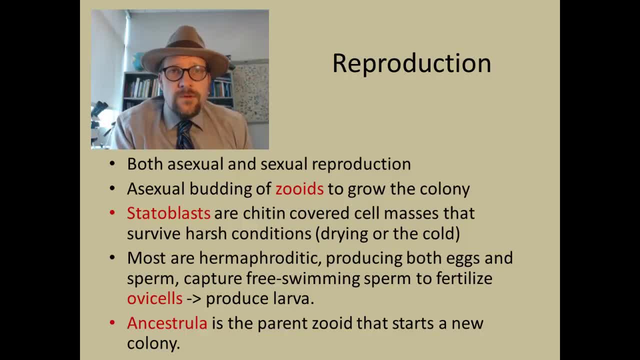 establishment of new colonies. Some zooids, secrete statoblasts, chitin-covered cell masses that can cover zooids and allow them to survive harsh conditions such as drying out or cold. Most zooids are hermaphroditic, which means they produce both eggs and eggs. 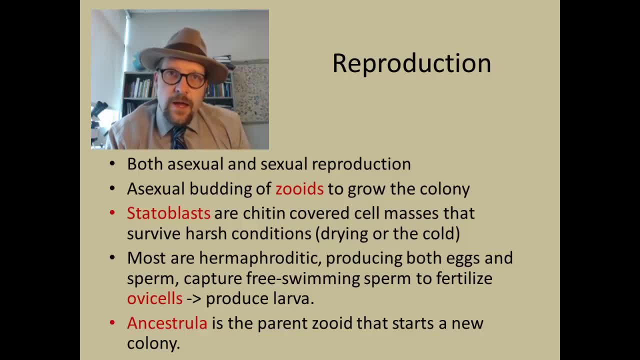 The sperm is free-swilling and will go about fertilizing eggs located in the oval cells of some bryozoans. These fertilized eggs then produce a larvae, and these larvae can be released into the water with the hope that it will form a new colony. 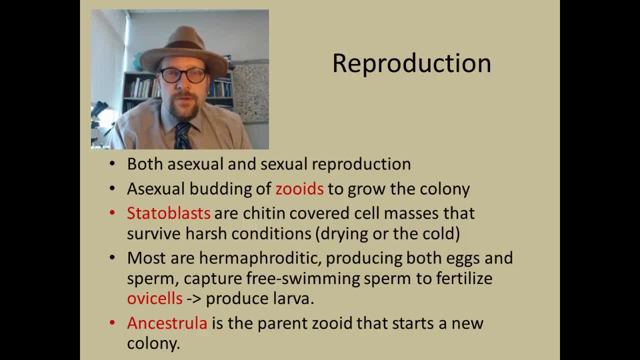 The parent larvae zooids form what is called the anstralia, or the first established zooid in a colony. Now, Given the anatomy of the colony, paleontologists can speculate on which of the zooicum represents the anstralia for the entire colony. 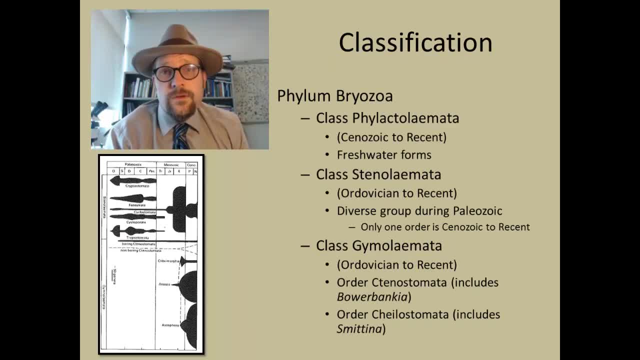 Let's now look at the classification of various groups of bryozoans. There are three classes: The Phenacolomata, which are the freshwater forms, and they have a fossil record that extends back to the Cenozoic. The Stenolomata have a diverse fossil record. 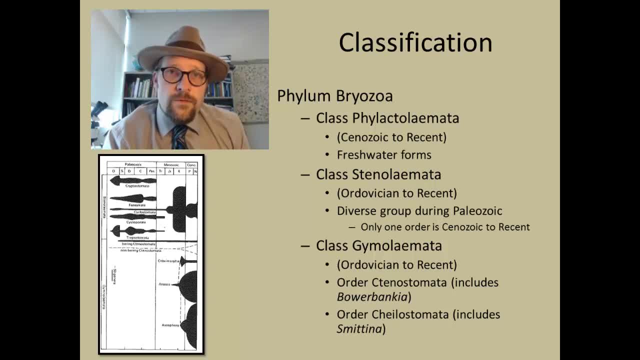 They were the most numerous during the Paleozoic, with a fossil record extending back to the Ordovician. The final class is the Gymlomata, with a fossil record extending back to the Ordovician and includes both the brown Bancarii and Smetellae. 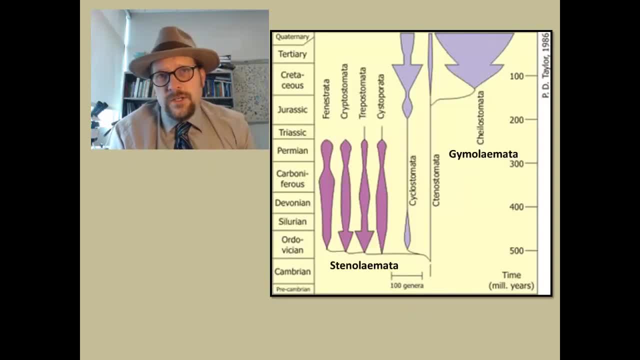 Note that bryozoans don't appear until the Ordovician, despite their primitive nature. The Cnidarians predate bryozoans, but during the Ordovician and into the Permian bryozoans remain very common in the fossil record. Now let's take a look at the various groups of the marine bryozoans, the Stenolomata and the Gymlomata. The Stenolomata have four extinct groups that all died out at the Permian-Triassic boundary. 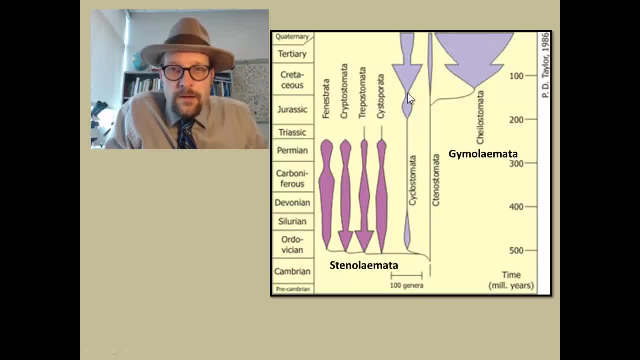 with one group, the Cyclostomata, that extends up through that boundary up into the Cenozoic. The Gymlomata, which is the Cynostomata, is a group that died out at the Permian-Triassic. 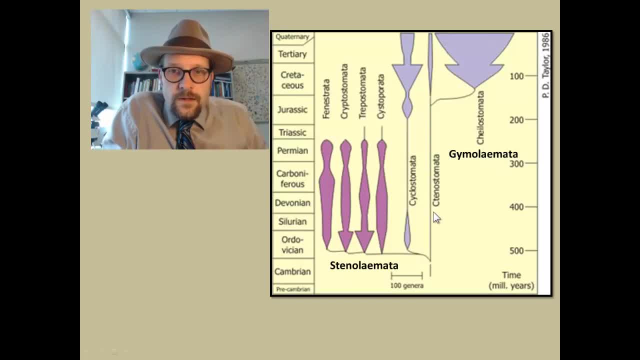 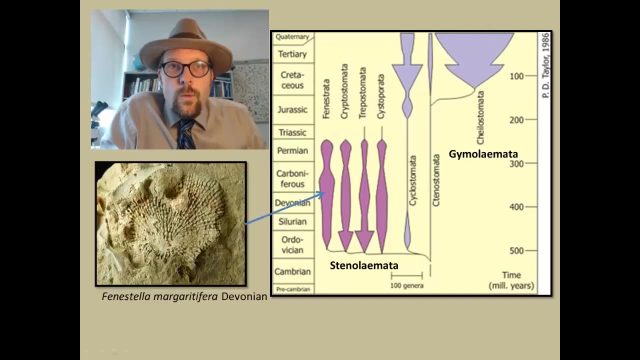 boundary, with one group, the Cyclostomata, that extends up through that boundary up into the Cenozoic. The Stenolomata includes the Tiniostomata that has a fossil record that goes back to the Ordovician, and the more common, the Sheleostomata, which is known mostly since the Late Cretaceous. 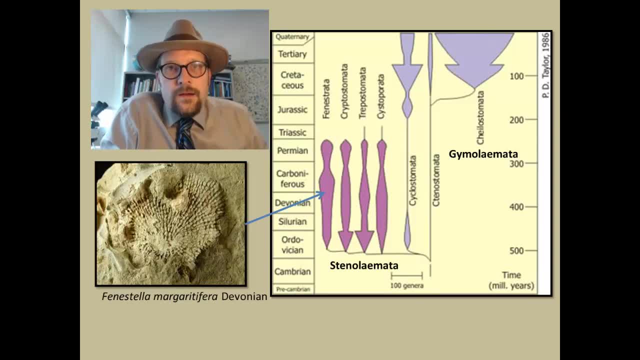 One of the most common extinct Stelomata Laumata is the Finestria Finestella. that can be recognized based on its fan-like lacy growths. The Finestrata also contains some really weird bryozoans. 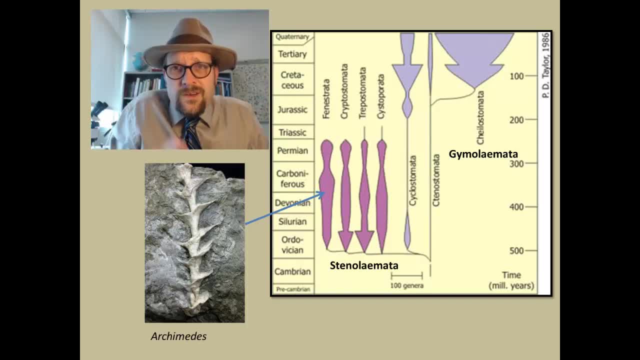 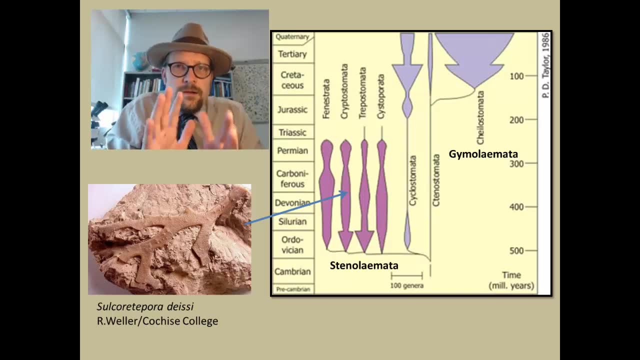 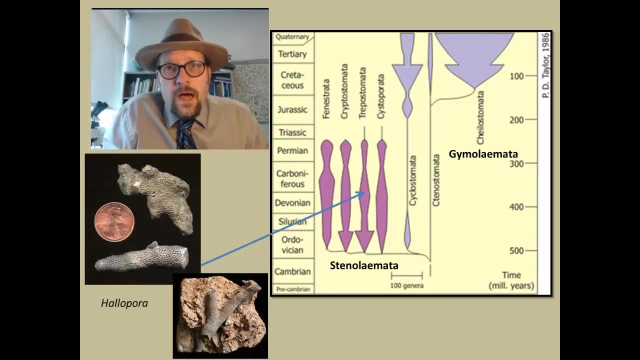 The Finestrata also contains some really weird bryozoan fossils. These include the Corkscrew Archimedes. The Extinct Clipostomata are branching bryozoans that have broad and fan-like structures. The Treptostomata include common branching or twiggy bryozoans. the Halopora recognized 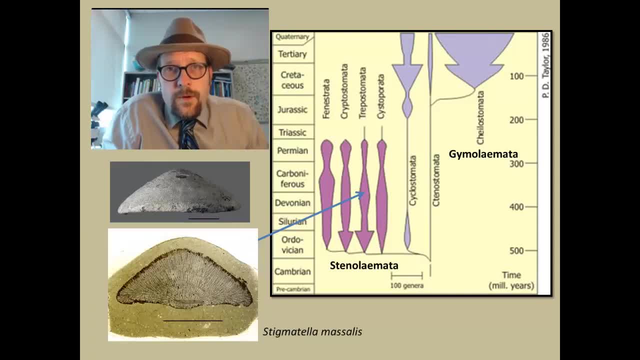 by the tiny zoacum. Some members of the Triptostomata form disk-like shapes and they have tiny perforations that extend into the interior of the colony like stones. Some members of the Triptostomata form disk-like shapes and they have tiny perforations that. 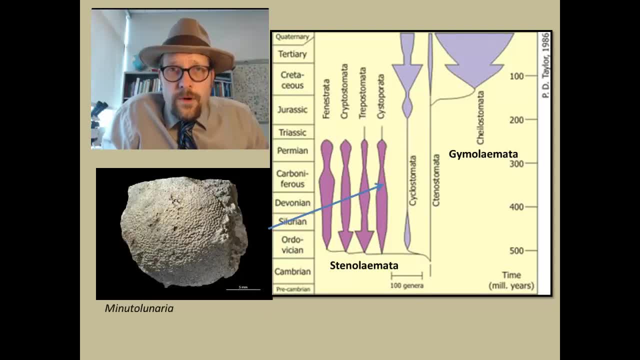 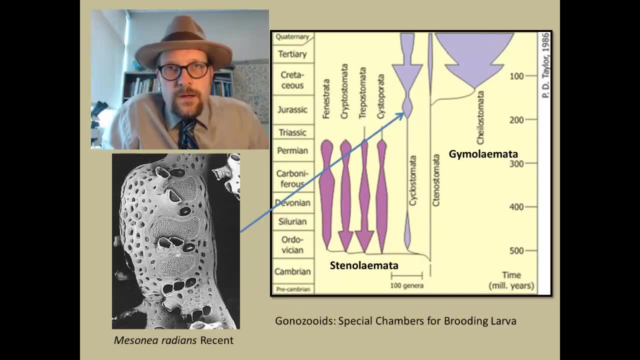 extend into the interior of the colony like stones. Some members of the Triptostomata form disk-like shapes like stones. The Cystopora are similar in being large colonies, often encrusting in irregular shapes. The Cyclostomata include the recent Misanella and are different in that. this group has what 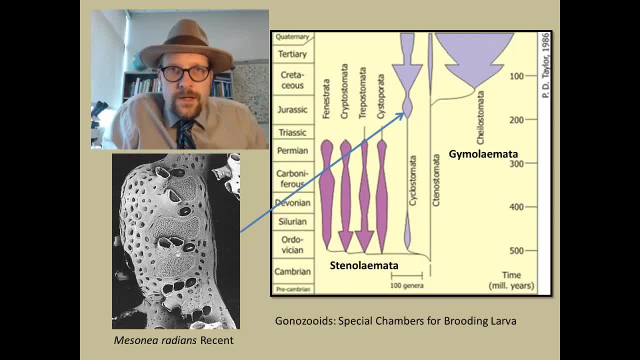 are called gonazoids. These are large openings for brooding larvae within the ova cell. Gonazoids can be distinguished from the more typical. smaller openings for the Lophophore. The smaller openings are for the Lophophore. The smaller openings are for the Lophophore. 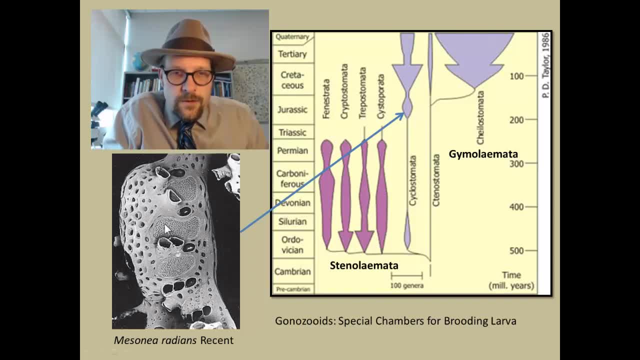 The smaller openings are for the Lophophore. A larger opening for bronchiola quarticinae is for the gonazoids that open up and releases the larvae. A larger opening for bronchiola quarticinae is for the gonazoids that open up and releases.